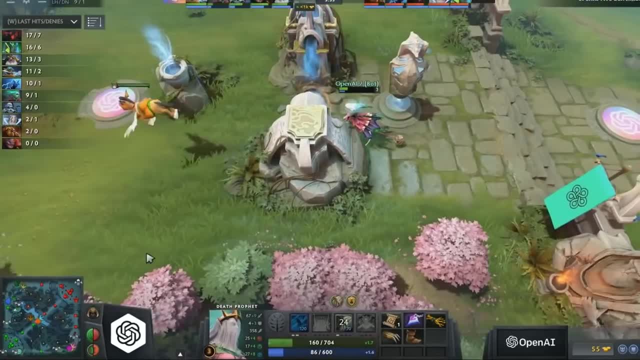 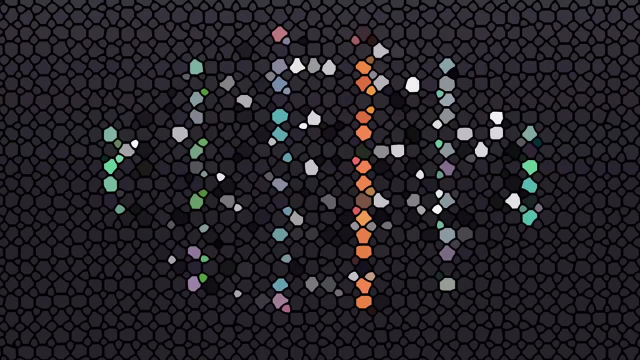 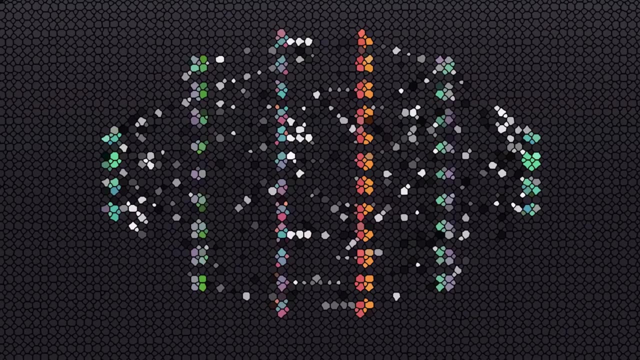 So what can we do when we want to step up our game from a simple toy environment like Frozen Lake to something more sophisticated? Well, rather than using value iteration to directly compute Q-values and find the optimal Q-function, we instead use a function approximator to estimate the optimal Q-function. 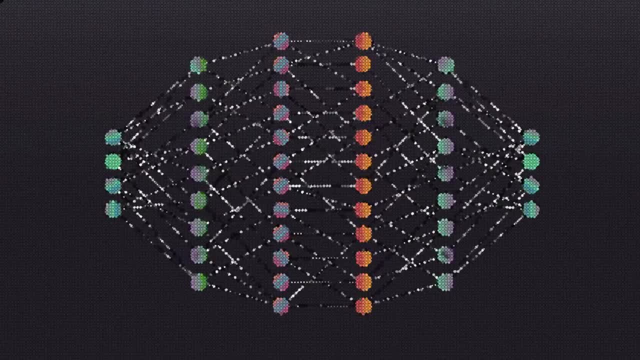 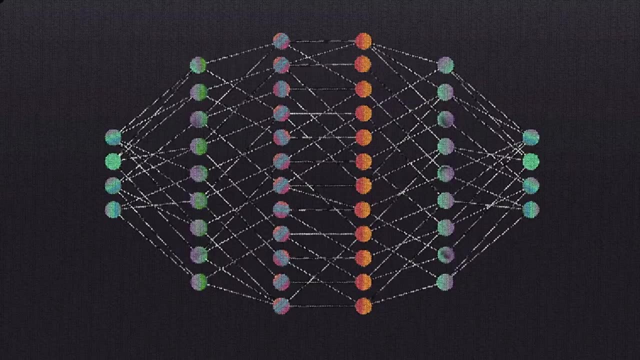 Hmm, well, you know what can do a pretty darn good job at approximating functions: Artificial neural networks. We'll make use of a deep neural network to estimate the Q-values for each state action pair in a given environment and in turn, the network will approximate the optimal Q-value. 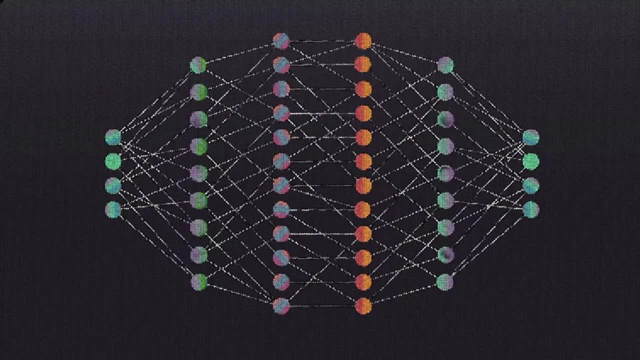 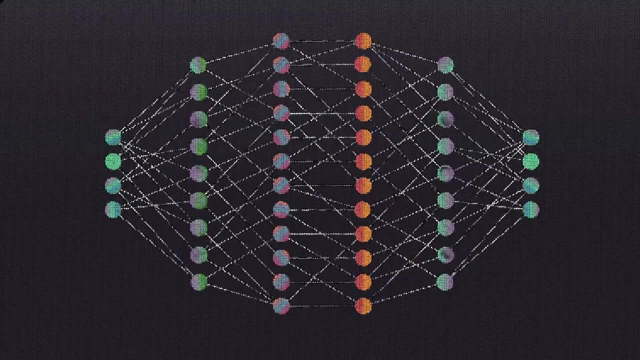 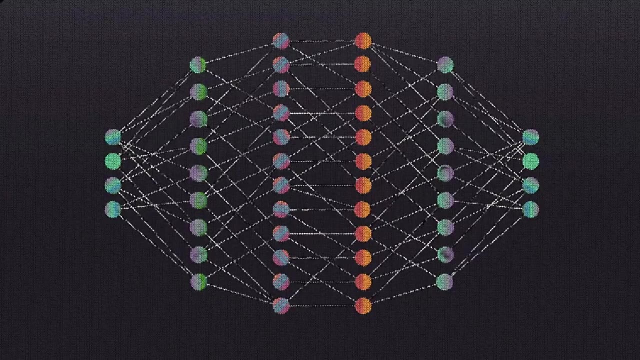 The optimal Q-function. The act of combining Q-learning with a deep neural network is called deep Q-learning, and a deep neural network that approximates a Q-function is called a deep Q-network or DQN. Let's break down how exactly this integration of neural networks and Q-learning works. 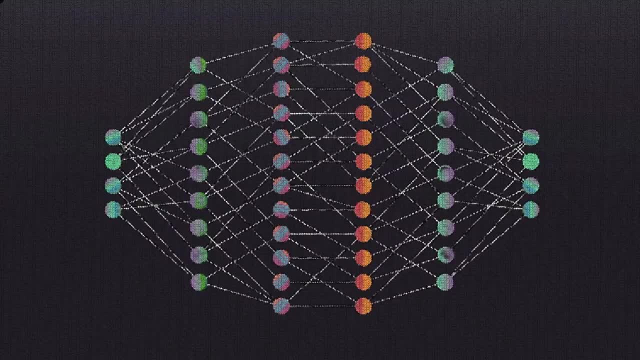 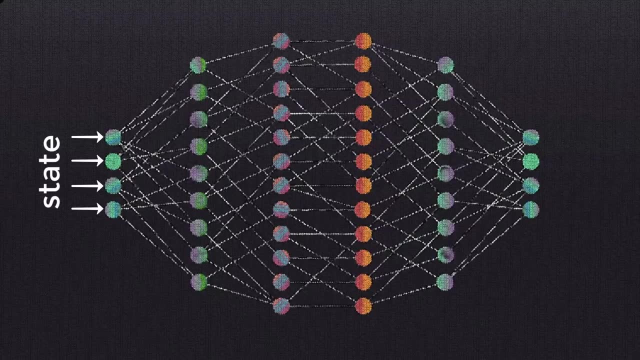 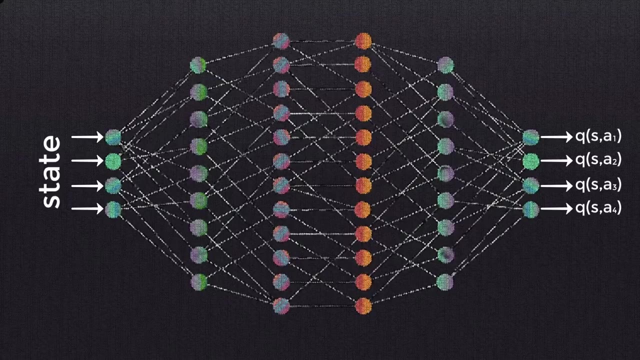 We'll first discuss this at a high level and then we'll get into all the nitty-gritty details. Suppose we have some arbitrary deep neural network that accepts states from a given environment as input. For each given state input, the network outputs estimated Q-values for each action that can be taken from that state. 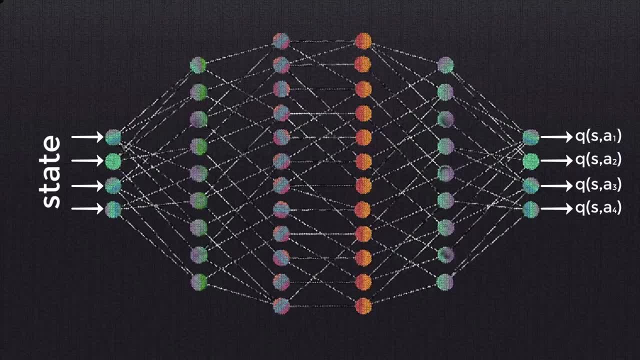 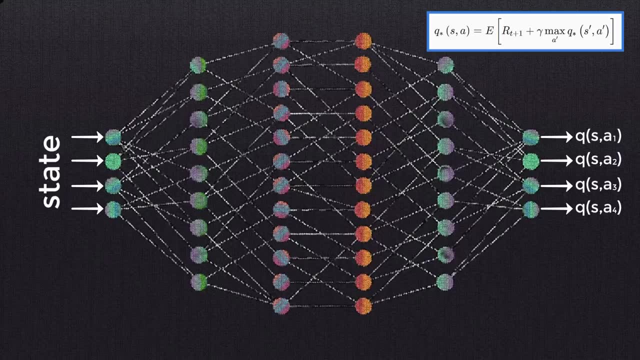 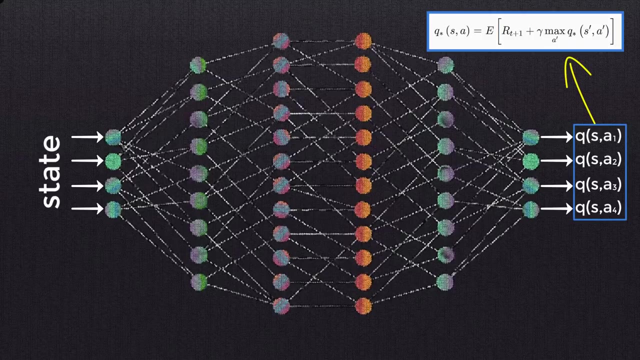 The objective of this network is to approximate the optimal Q-function, and remember that the optimal Q-function will satisfy the Bellman equation that we covered previously. With this in mind, the loss from the network is calculated by comparing the outputted Q-values to the target Q-values from the right-hand side of the Bellman equation. 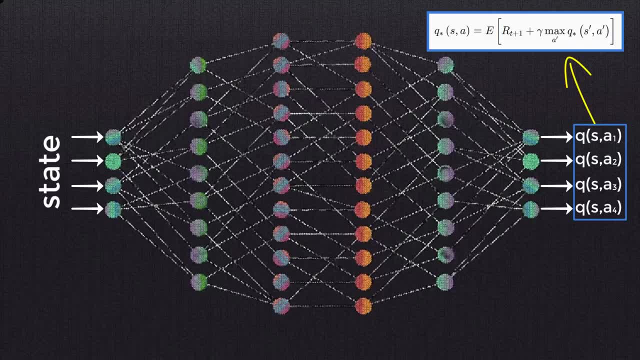 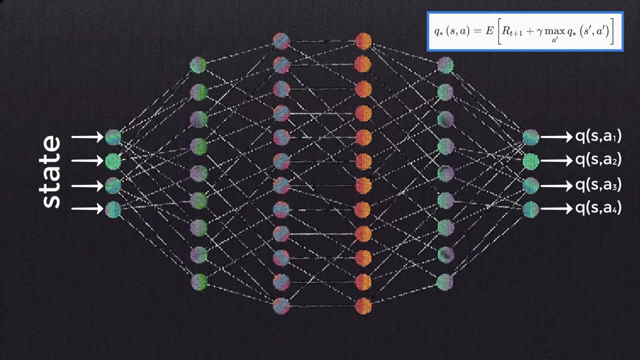 and, as with many standard networks, the objective here is to minimize this loss. After the loss is calculated, the weights within the network are updated via stochastic gradient, descent and backpropagation. again, just like with any other typical network. This process is done over and over again for each state in the environment. 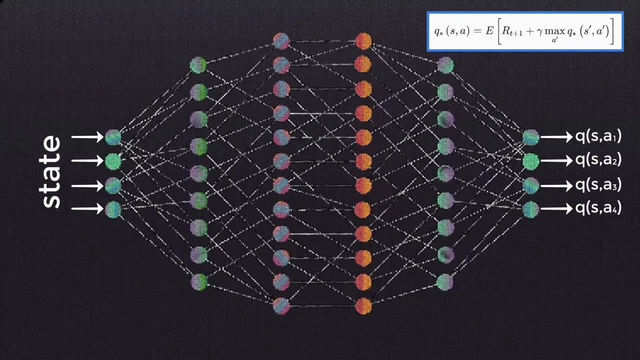 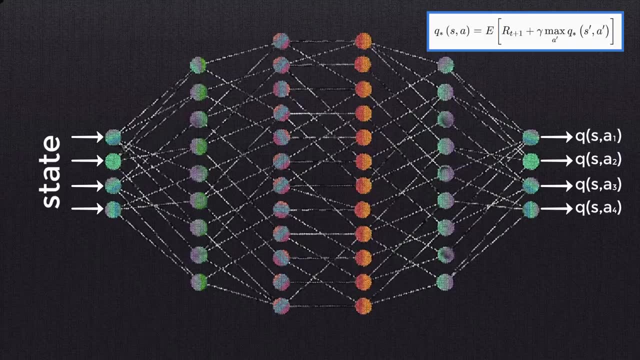 until we sufficiently minimize the loss and get an approximate optimal Q-function. So take a second now to think about how we previously used the Bellman equation to compute and update Q-values in our Q-table in order to find the optimal Q-function. 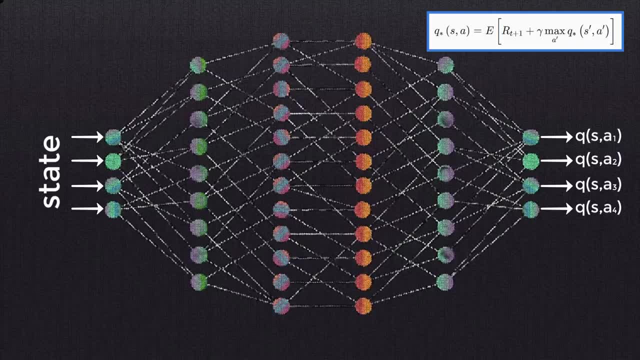 Now with deep Q-learning, our network will make use of the Bellman equation to estimate the Q-values to find the optimal Q-function. So we're still solving the same general problem here, just with a different algorithm. Rather than making use of value iteration to solve the problem, 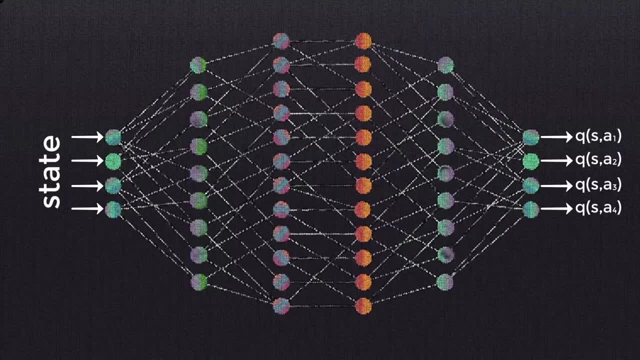 we're now using a deep neural network. Alright, we should now have a general idea about what deep Q-learning is and what, at a high level, the deep Q-network is doing. Now let's get a little more into the details about the network itself. 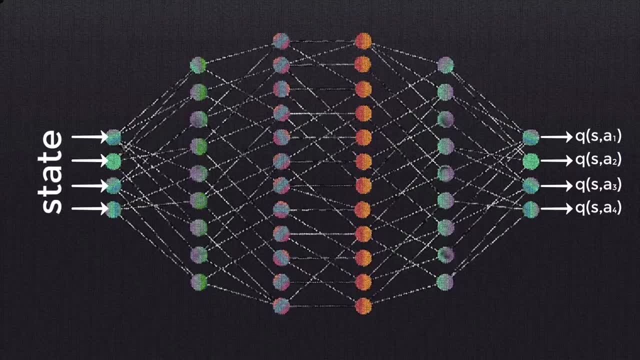 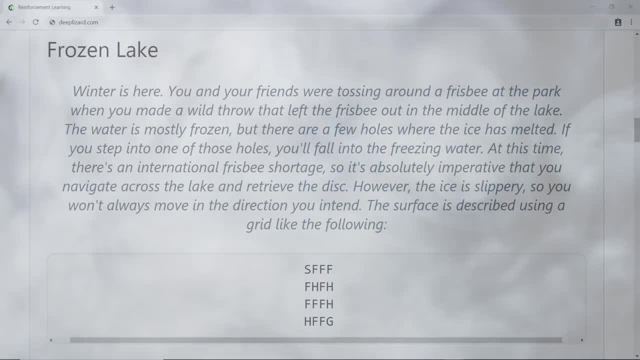 So we discussed earlier that the network would accept states from the environment as input. Thinking of the game Frozen Lake that we played last time, we could easily represent the states of this environment using a simple coordinate system from the grid of the environment. If we're in a more complex environment, though, like a video game, for example, 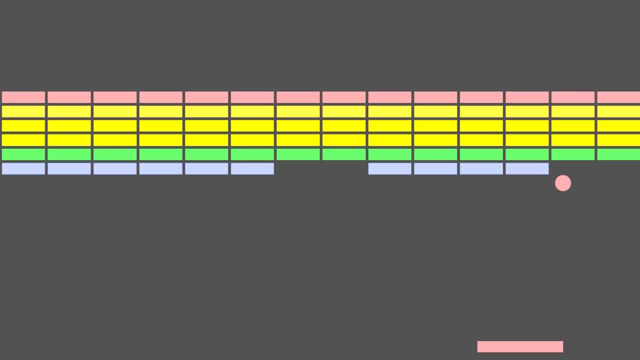 then we'll use images as our input. Specifically, we'll use still frames that capture states from the environment as the input to the network. The standard pre-processing done on the frames usually involves converting the RGB data into grayscale data, since the color in the image is probably usually not going to affect the state of the environment. 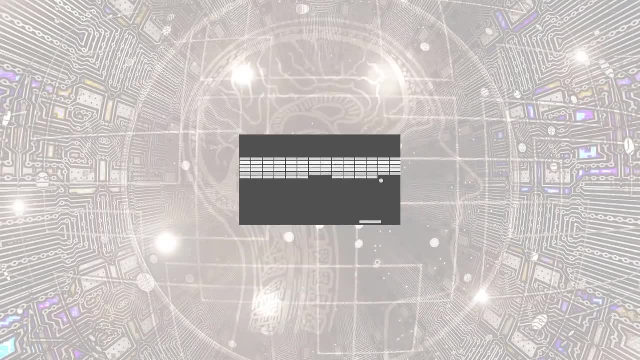 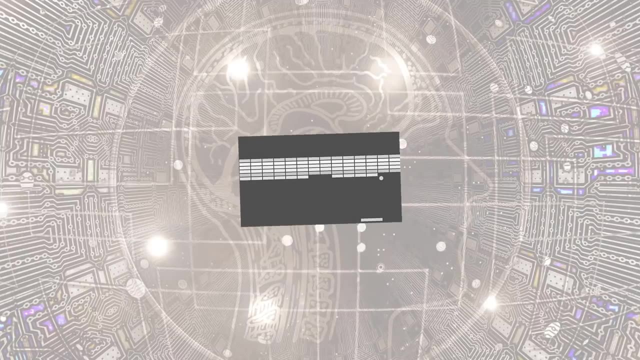 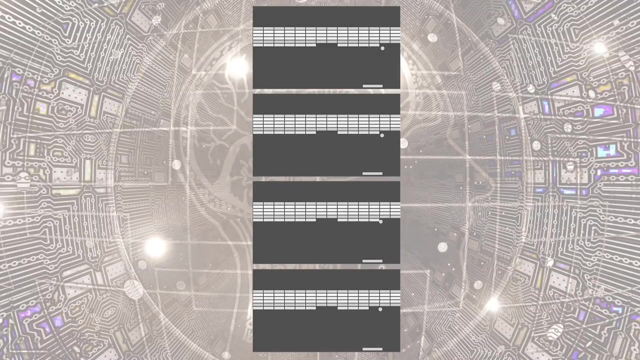 Additionally, we'll typically see some cropping and scaling as well, to both cut out unimportant information from the frame and shrink the size of the image. Now, actually, rather than having a single frame represent a single input, we usually will use a stack of a few consecutive frames to represent a single input. 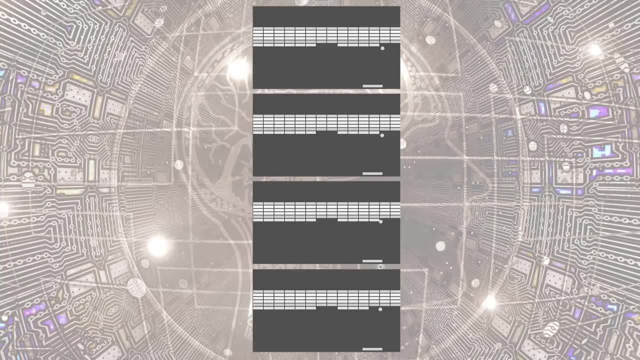 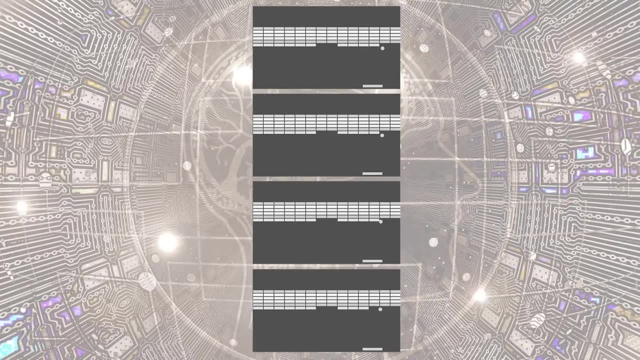 So we'd grab, say, four consecutive frames from a video game. We'd then do all the pre-processing on each of these four frames- we mentioned earlier- the grayscale conversion, the cropping and the scaling- And then we'd take the pre-processed frames and stack them on top of each other. 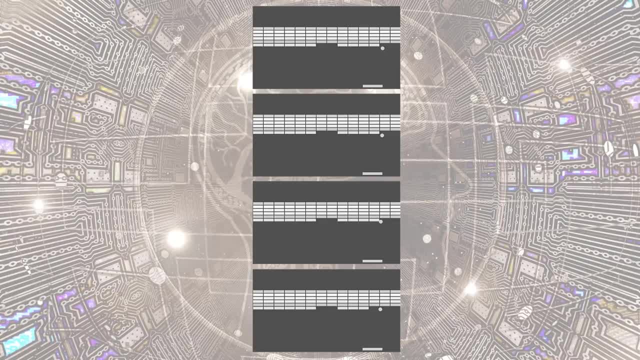 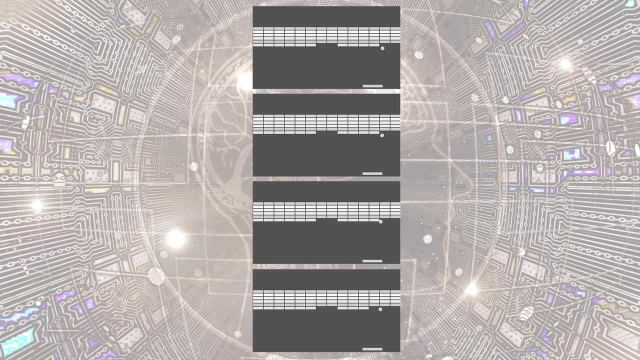 in the order of which they occurred in the game. We do this because a single frame usually isn't going to be enough for our network, or even for our human brains, to fully understand the state of the environment. For example, by just looking at this single frame from the Atari game Breakout. 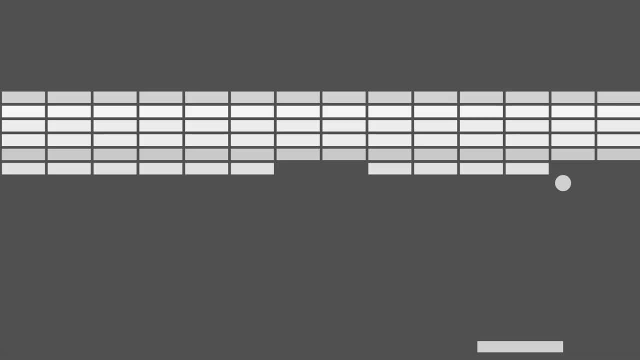 we can't tell if the ball is coming down to the paddle or going up to hit the block. We also don't have any indication about the speed of the ball or which direction the paddle is moving in. If we look at our four consecutive frames, though, 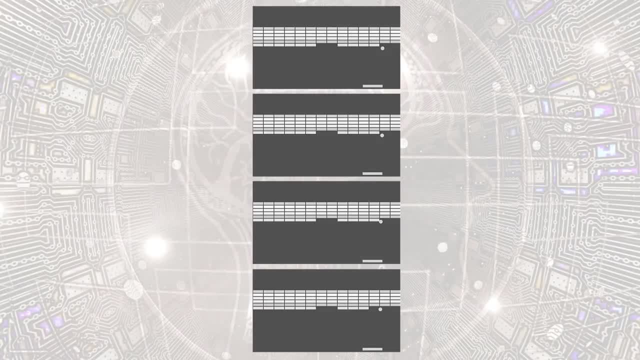 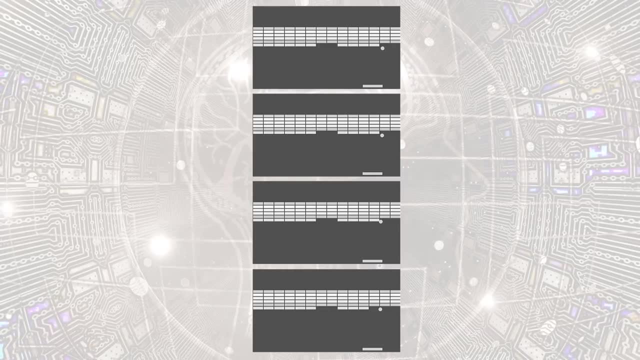 then we have a much better idea about the current state of the environment, because we now do indeed have information about all of these things that we didn't know, with just a single frame. So the takeaway is that a stack of frames will represent a single input. 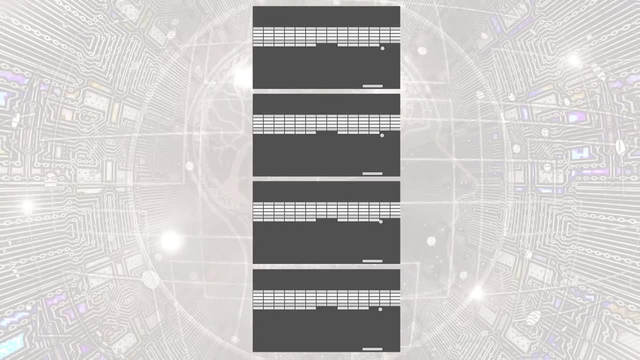 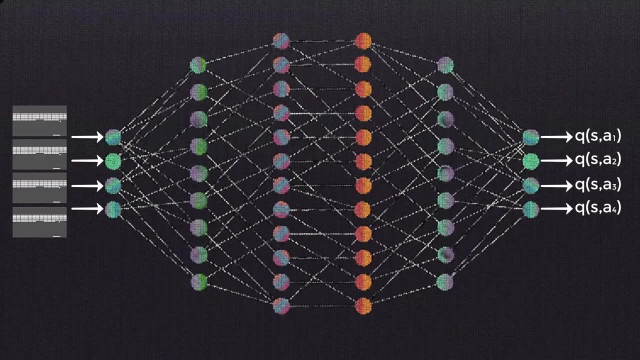 which represents the state of the environment. Now that we know what the input is, the next thing we need to address is the inner workings of the network, the layers. Well, really, we're not going to see much more than we're used to seeing. 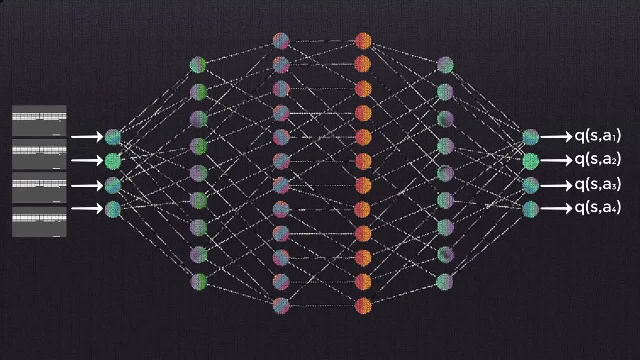 with any other network we've already covered, Like seriously many DeepQ networks are purely just some convolutional layers followed by some nonlinear activation function, and then the convolutional layers are followed by a couple fully connected layers and that's it. 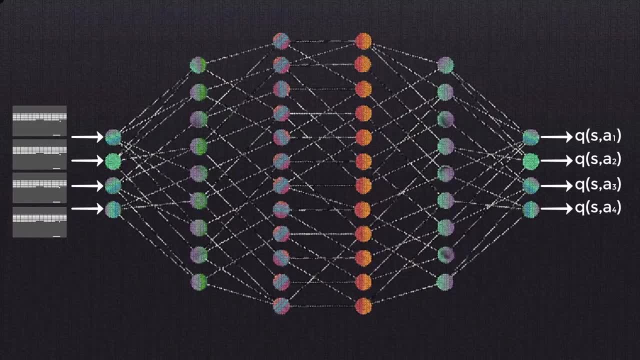 So the layers used in a DQN are nothing new and nothing to be freaked out about. If you do need a crash course or a refresher on convolutional neural networks or on neural networks in general, then be sure to check out the Deep Learning Fundamentals series. 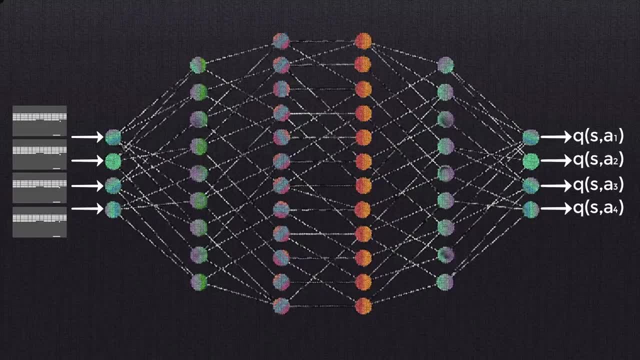 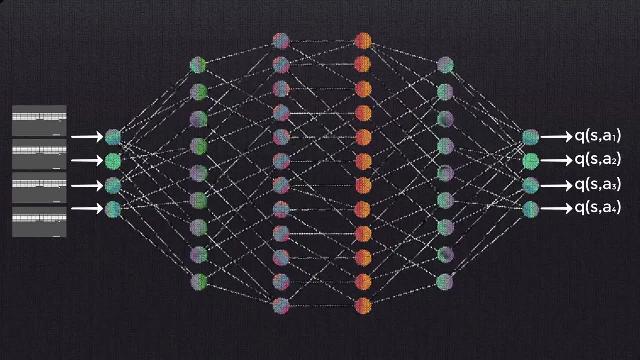 The last piece of the network to discuss is the output. The output layer will be a fully connected layer and it will produce the Q value for each action that can be taken from the given state that was passed as input, For example, suppose, in a given game. 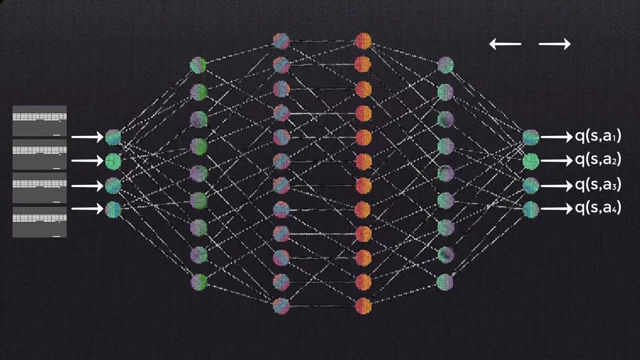 the actions we can take consist of moving left, moving right, jumping and ducking. Then the output layer would consist of four nodes, each representing one of the four actions. The value produced from a single output node would be the Q value associated with taking the action that corresponds to that node. 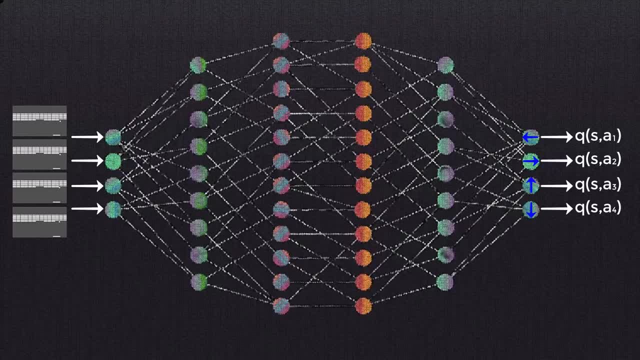 from the state that was supplied as input to the network. We won't see the output layer followed by any activation function, since we want the raw, non-transformed Q value from the network. Alright, so now we know what deep Q learning and deep Q networks are. 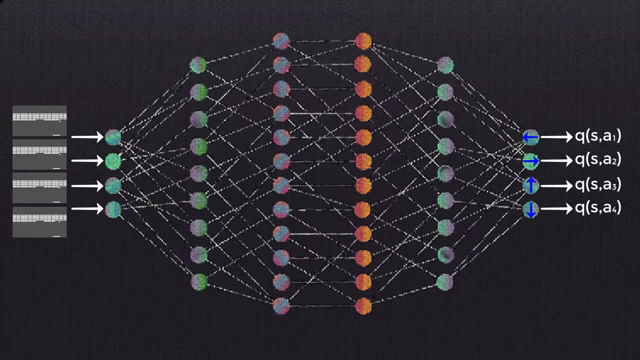 what these networks consist of and how they work. I know when I was originally learning about DQNs, I was prepared to learn some type of new and mysterious neural network and was pretty surprised when I found out that really there was nothing new about the network at all. 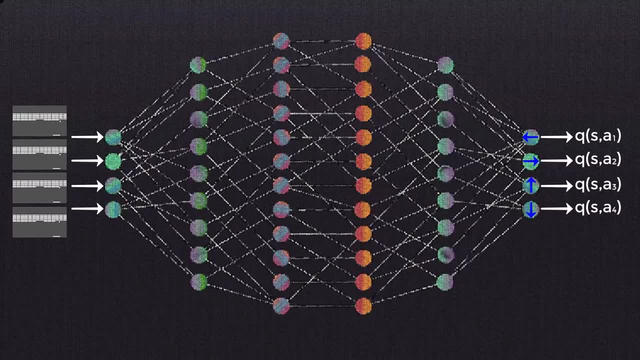 Instead, we were just utilizing a CNN to solve a different type of problem. Let me know in the comments if you're feeling the same way and stay tuned, because in the next video we'll continue discussing DQNs and dissect the training process. 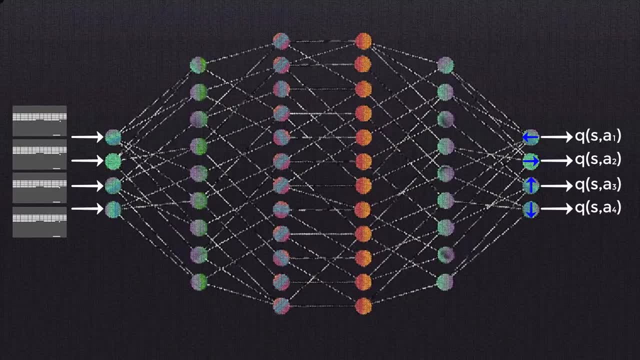 step by step to prepare ourselves to create and train our own DQN and code. Please leave a thumbs up to let us know you're learning, and be sure to check out the corresponding blog to this video, as well as the Deep Blizzard Hivemind, for exclusive perks and rewards. 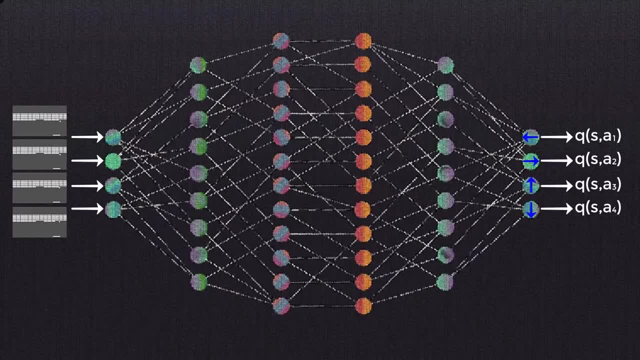 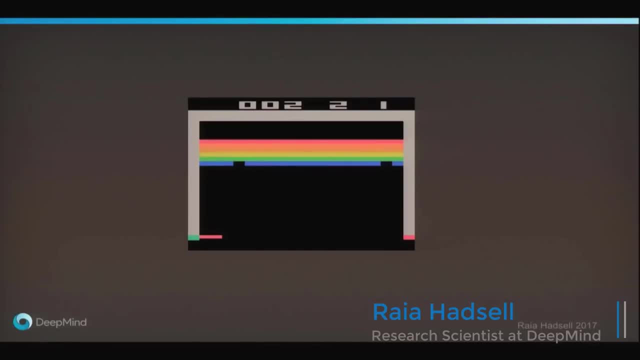 Thanks for contributing to Collective Intelligence and I'll see you in the next one. One particular game I can show to you is this game. It's an Atari game called Breakout. Those of you that are a child of the 70s or 80s. 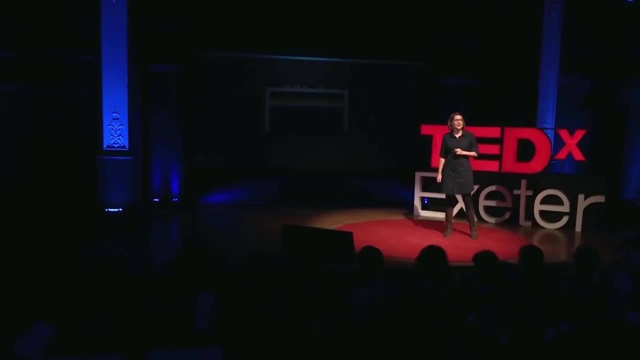 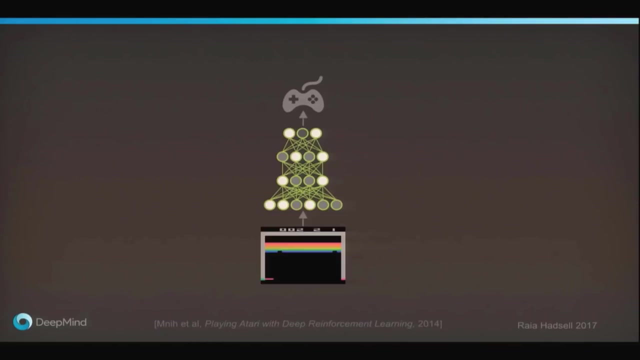 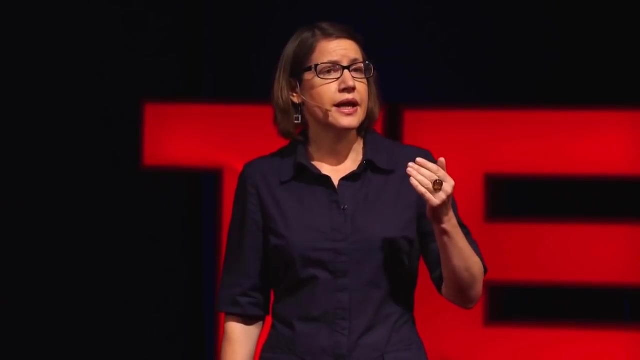 may remember it very well, maybe new to others of you, And the way an agent learns to play this game is by seeing the pixels on the screen, then making mathematical calculations which propagate through those millions of connections, layer by layer in the network, producing an action which is a command on the joystick. 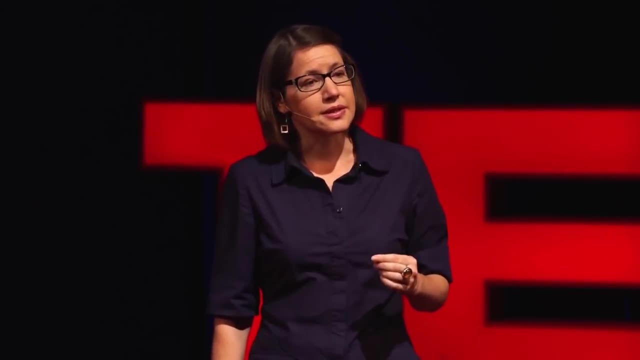 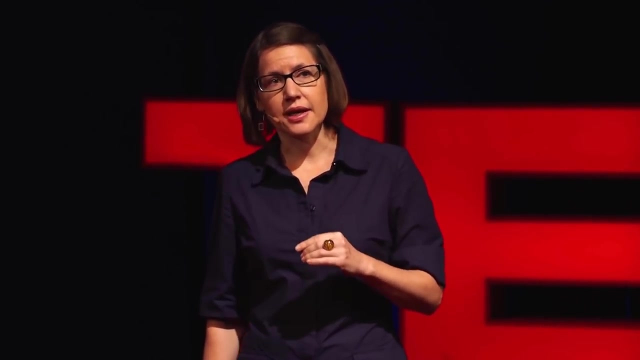 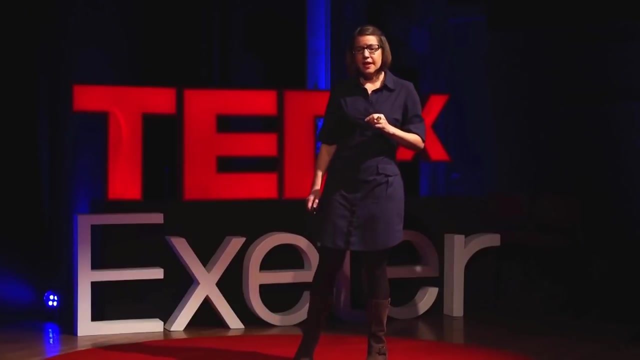 Now, if that action is good and results in the agent getting more points, more reward, then the learning algorithm reinforces that action by adjusting ever so slightly all of the millions of connections in that neural network. We can see how the behavior of the agent changes over time. 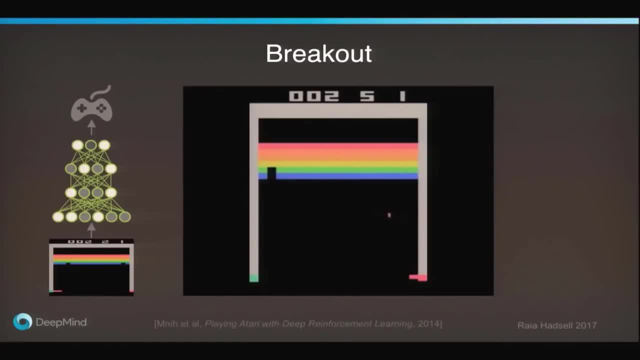 with its experience of the game. So at first, even after 100 games of experience, it's still pretty rubbish. It misses the ball all too often. But if it keeps on playing- after a few hours, 300 games- then it gets better and better. 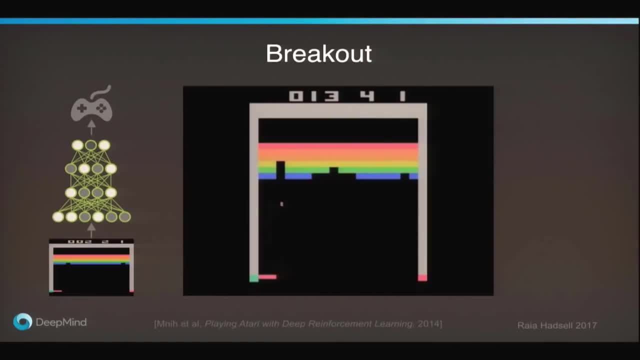 At this point it's at about human ability. It can return the ball, keep alive for a long time. If we let it keep on learning, then after a few more hours and a lot of games of experience, then it gets really good. 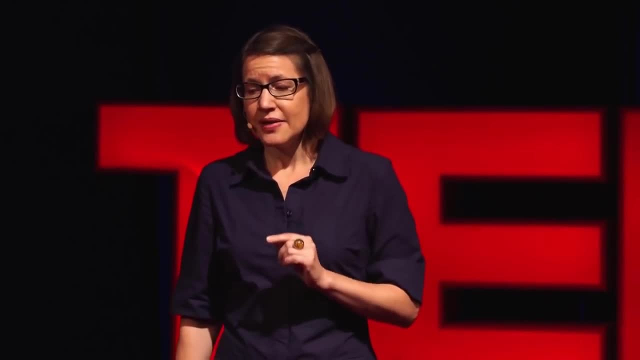 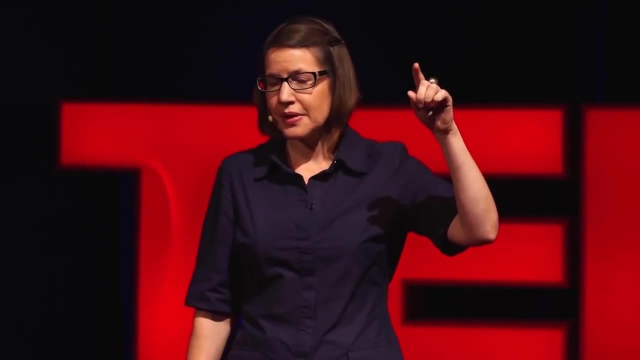 It gets better than a human because it learns how to do this trick called tunneling, That is, systematically send the ball to the sides of the wall so that it bounces around on top and the agent has less work and more reward. The learning algorithm doesn't just work. 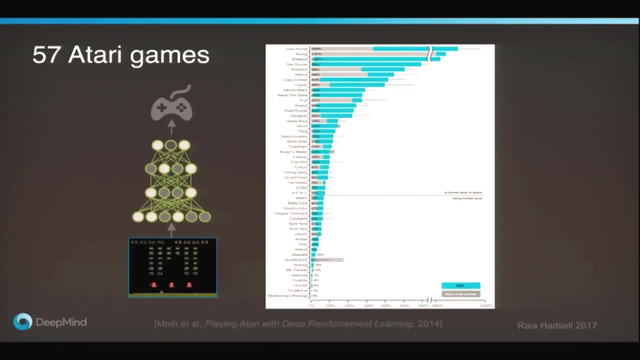 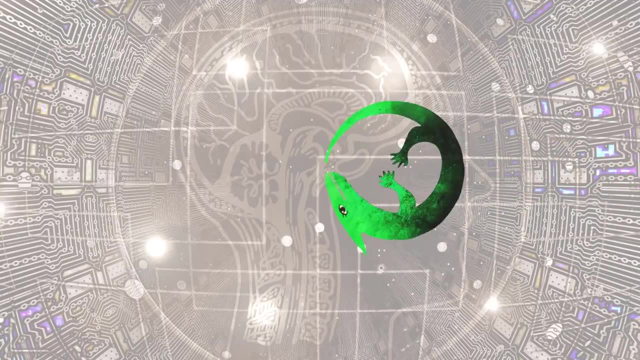 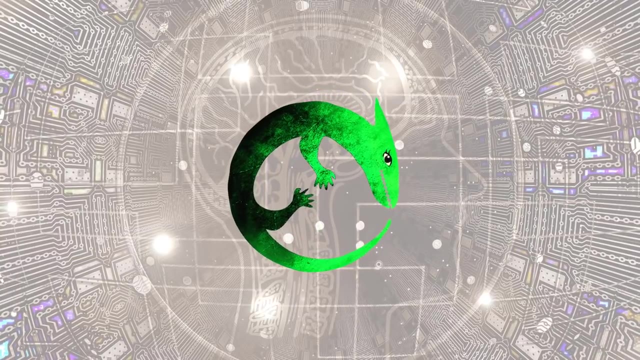 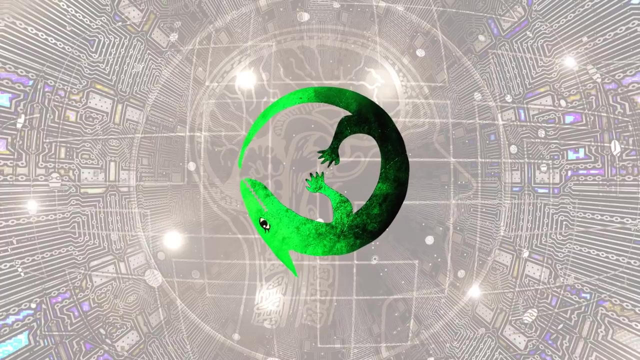 It works on most of the 57 games that we've tried it on and achieves superhuman level of play at most of them. Subtitles by the Amaraorg community.